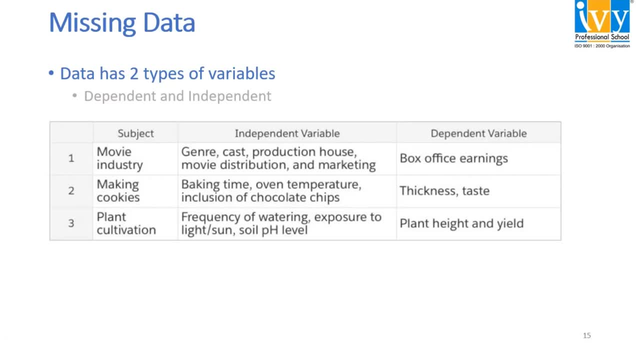 All these three are not correlated to each other, but they are independent. What is dependent is the thickness and taste of the cookies. The third we can see is plant cultivation, the frequency of watering, exposure to light or sun and the soil pH level. 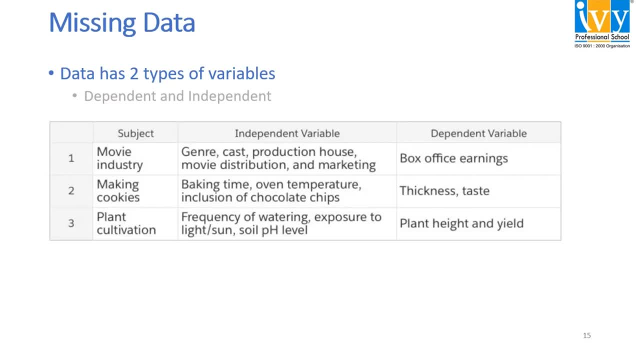 These three are the independent variables. What is dependent is plant height and heat. So this way, let's have a look at the data And see what we can do with the missing data. It may be missing in either or both type of variables. 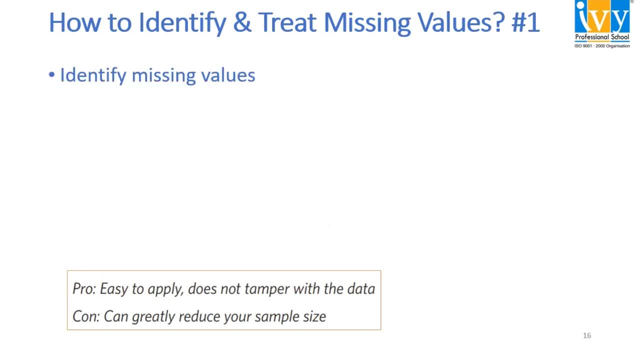 But how to identify and treat missing values? To identify the missing values, count the total number of values in each column and then if the number of record is greater than the number of value, then definitely these are the missing values. so let's have a look at the data set. so 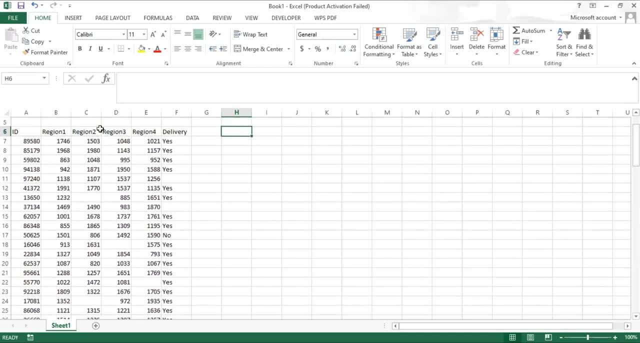 as we can see in this data set, there is an ID, there are four regions and then there's a delivery column. so how can we find if these data have missing values or not? firstly, the thing that we are going to see is that in this data ID, 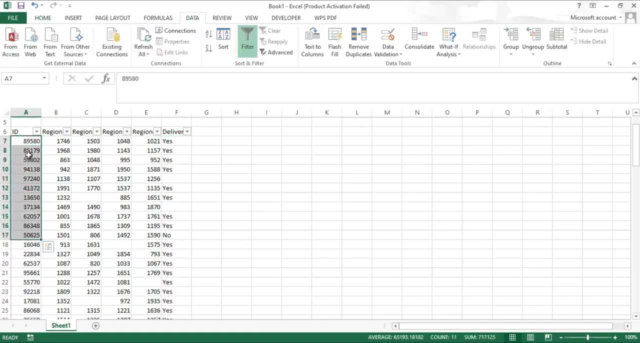 plays a very major part. it must definitely have unique values and must not have any missing values, otherwise the row will be completely discarded, because there's no point of keeping an empty ID with its region and the delivery data. so I have filtered the data and let's see if it has blank rows. 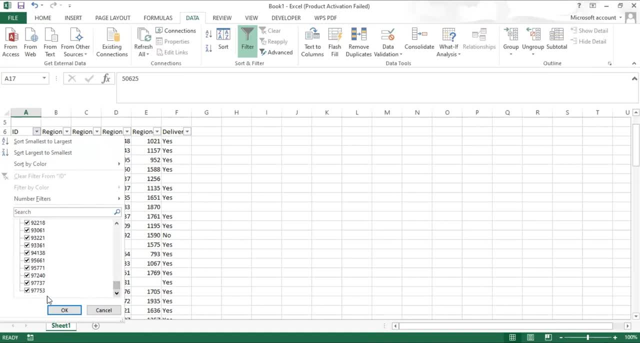 scrolling down, we can see that there are no blank rows. if a column has blank rows, it appears at the end of the filter. so we go back. we go to the region column and see if there are blanks. so yes, there are blank. let's go to region 2. 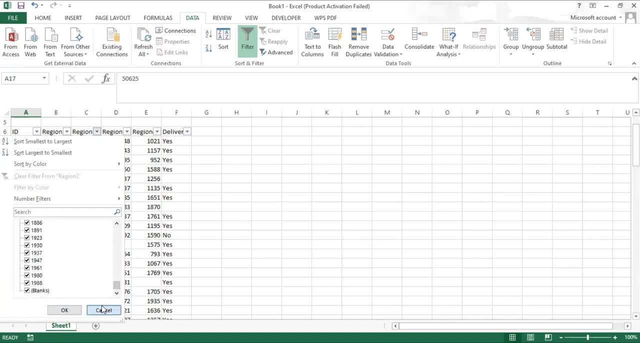 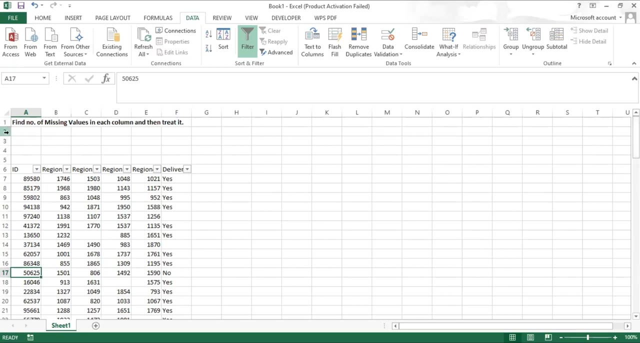 so blanks are there. region 3: we can see there's a blank. region 4: yes, blanks are there. and also in the delivery part there are blanks. so first we'll see, we'll work on the rows and then we'll go to columns, since the ID column has all the 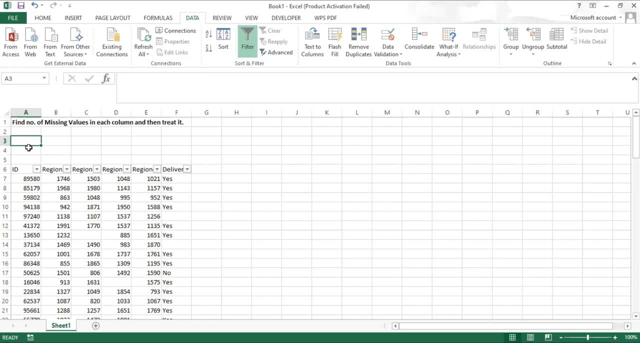 records. so what we'll do next is we'll go to the ID column and then we'll go to the rows, and then we'll go to the records, and then we'll use the count, a function, to calculate the total number of records over here. this will give us the accurate record. it appears that 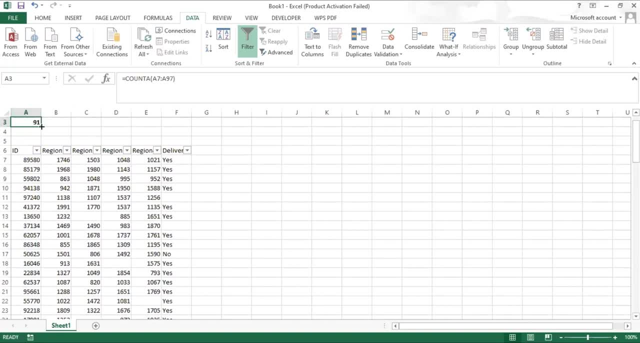 there are 91 records over here. the same can be done for the rest, and we see change in values in the rest of the records. after doing this, what we can do is change in values in the rest of the records. after doing this, what we can do is: 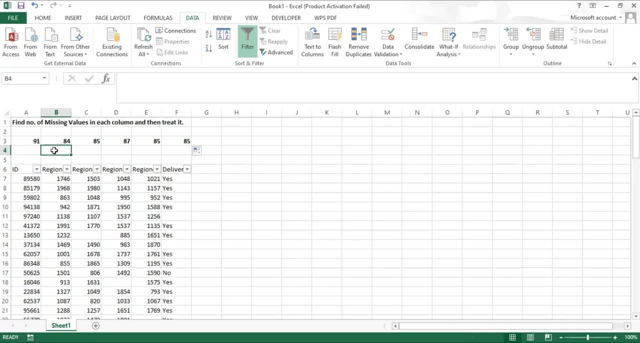 we can see the percentage difference or the percentage of missing values for each column. But doing that, what we'll do is I'll use a formula which will be one minus the number of missing values divided by keeping this fixed. So for all the columns, I'll go back. 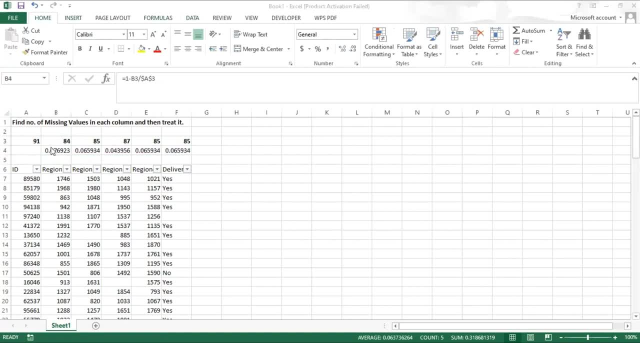 to the Home tab And what we can see here is missing values are 8%, 7,, 4,, 7% and 7%. Now, whenever all the records have more than 30% of the missing values, what we do is we: 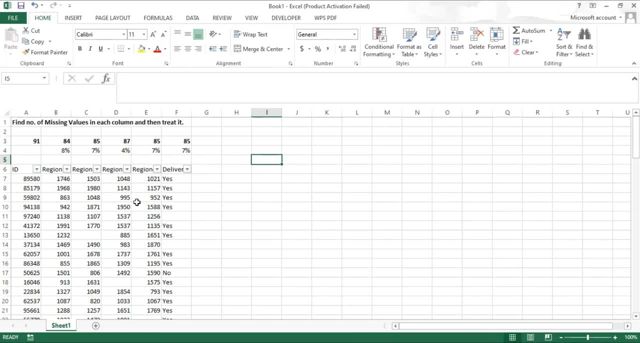 discard those records, that is, we delete the rows. But since these are very less percent, what we can do is we'll go back to the Home tab, And what we can do is we'll go back to the Home tab, And what we can do is we can change these things. So now let's have a 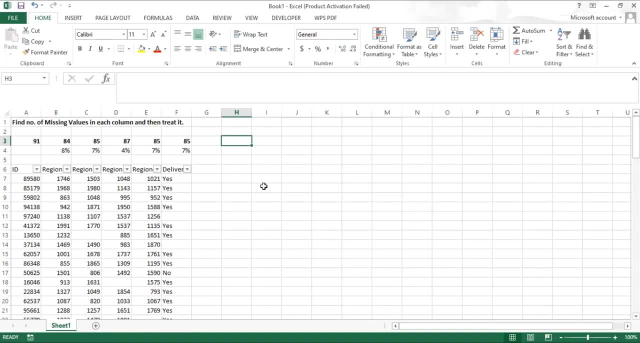 look at the column. For doing that and counting the accurate column numbers, I'll use count A on the headers And I'll do that. for the rest, We can see different values Now to find the percentage change. what we're going to do is we'll use equal. 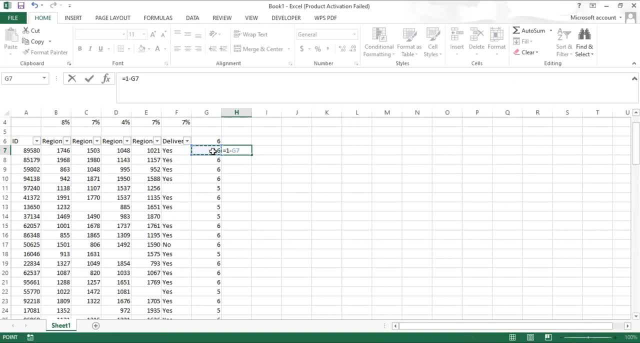 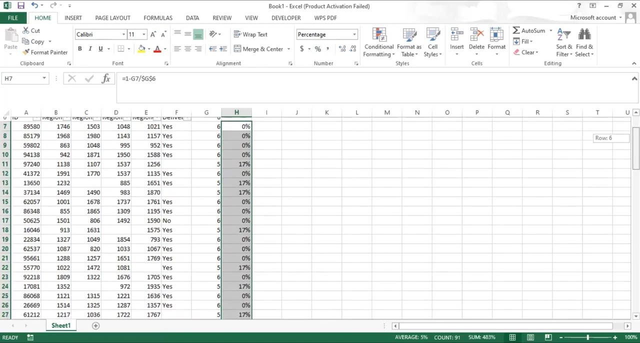 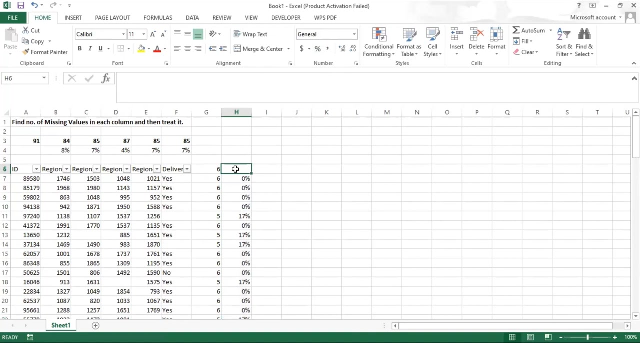 to one. minus this by keeping this as fixed. I use percentage and see 17.. So let's name these things. This column can be named as the missing count, And this can be pasted somewhere else. So what we'll do is and. 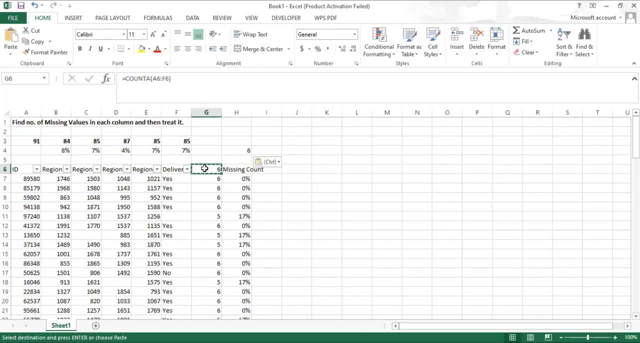 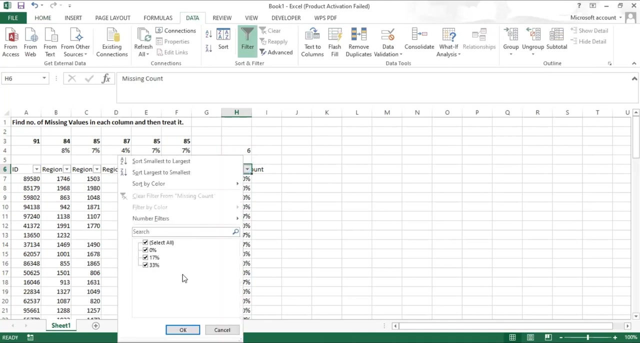 I'll name this column as the total count. After doing that, change my value over here to this, fix it And for the rest you're going to do the same. So calculating missing count, we see the maximum missing count is 33%. 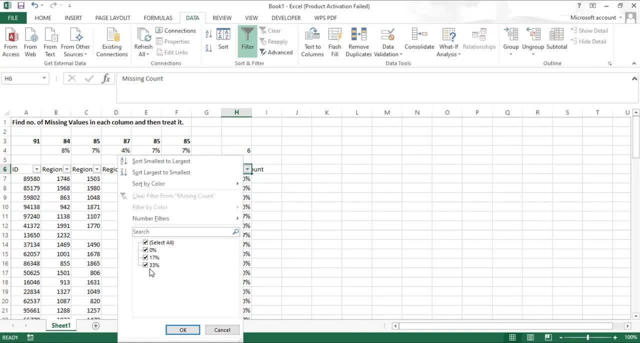 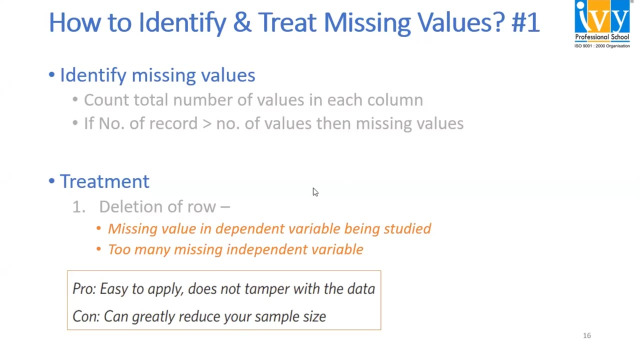 Had it been 50% or more, we could have discarded the column. That means we could have deleted the column. So what we have seen is that the treatment can be deletion of rows if there are more than 30% of the records are not there, or 50% in case of columns because we don't have. 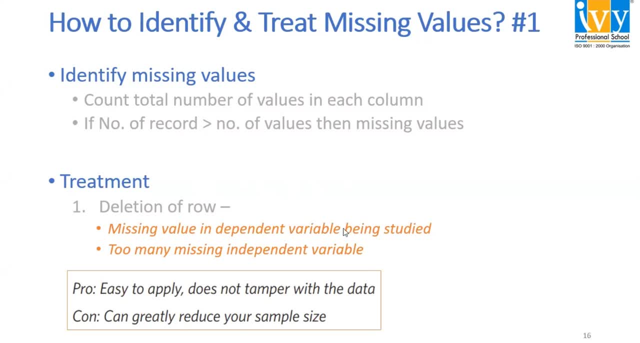 the data to work on, So we can delete it, And the pro is that it's easy to apply and does not tamper with the data. The con is that it can greatly reduce the size of the data on which we will work on. 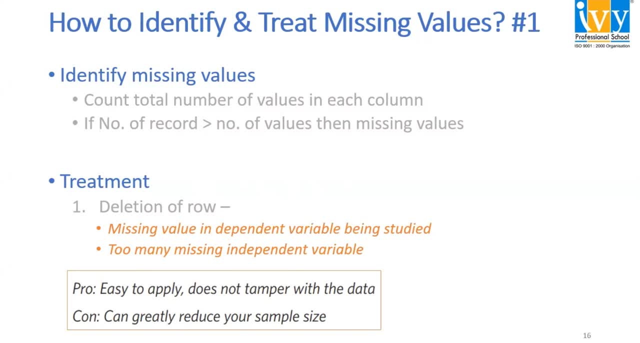 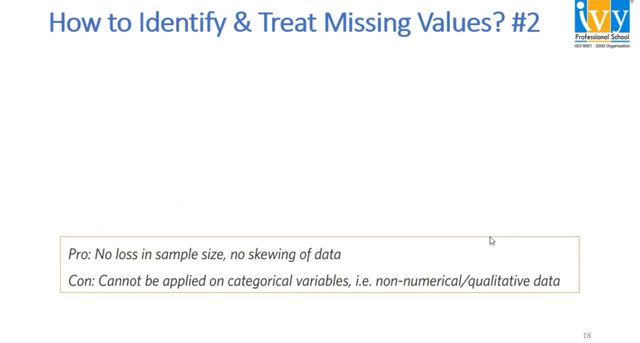 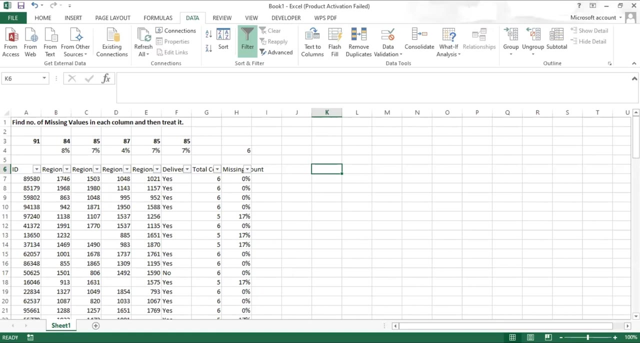 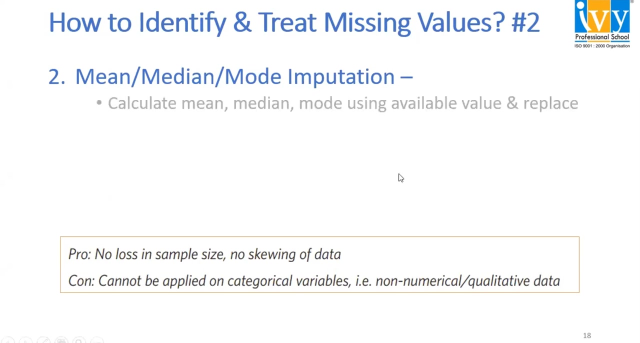 So now let's see how to identify and treat the missing values in a other way. So let's go back to our data. This is the data and we have seen that it has too many missing values. So let's see the methods. The methods are mean median and mode imputation, So we can 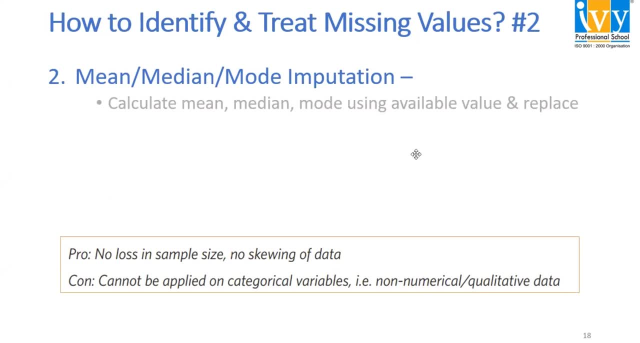 calculate mean median mode using available value and replace. Mean is commonly known as the average, which means summation of all the variables and dividing it by the total number of variables present. Median is the middle value in the range, and mode is the value which occurs most often in the range. Let's see how it works in case of our data. 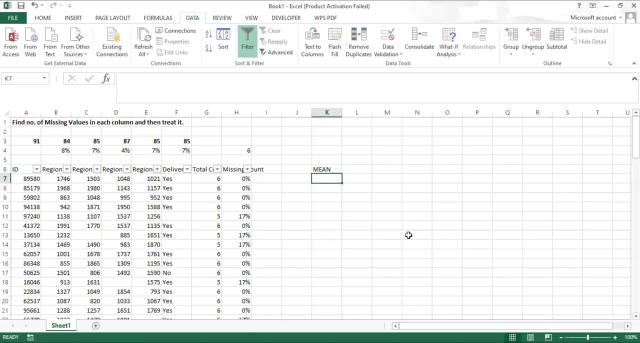 The first thing we are going to learn is using mean. In that case, let's go to region one and let's see how mean works over here. So I'll select all the cells. There's a gap in selection because there are too many missing values. 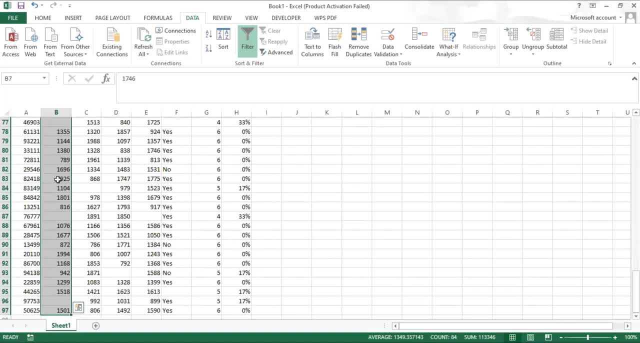 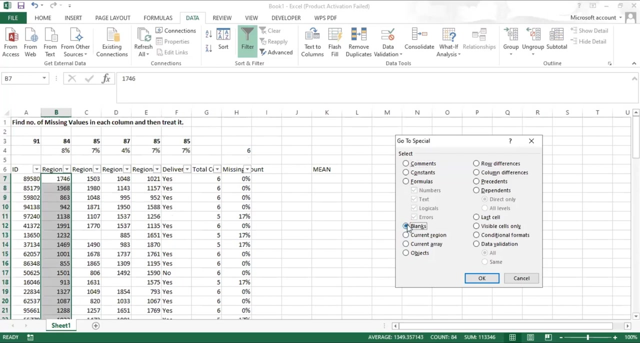 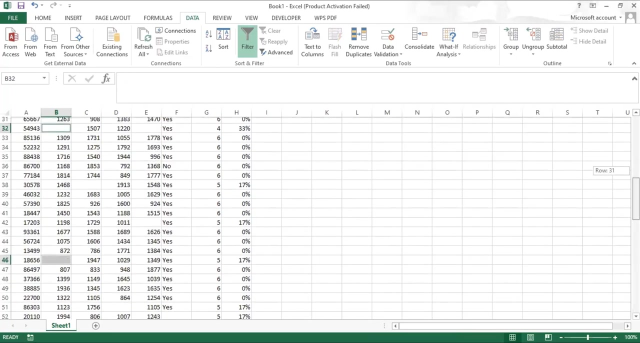 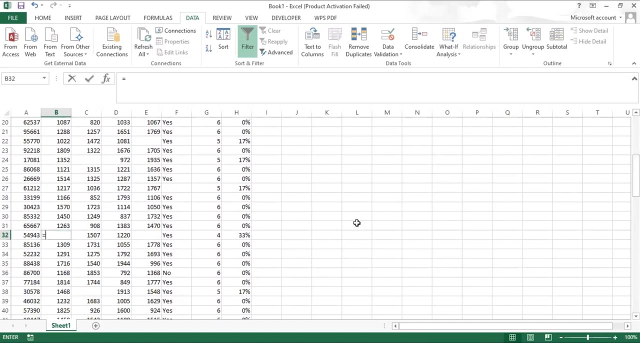 Okay, Now I'll press control G, I'll click on special and click on blanks. Click okay And see These are my blank cells. Now what to do? What I'll do is I'll simply write equal to average and select the entire. 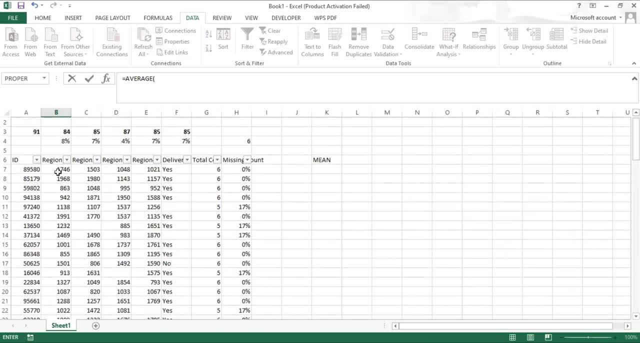 column. So I'd drag down. After that, I'll just create a column with the same name and I'll click on the column. I'll click on the column. Okay, Cool, dragging down. I've selected all the cells in a single column. 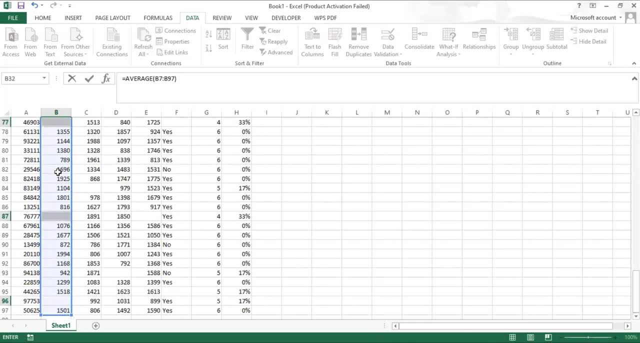 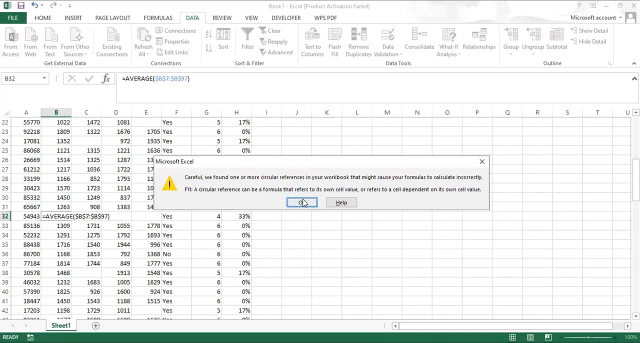 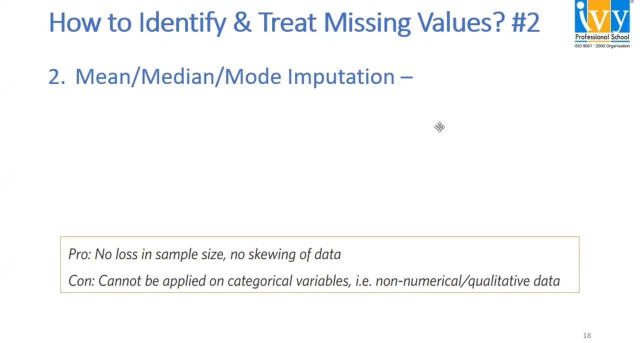 And click not on enter, but I'll click on control enter. What it will do is it will automatically clicking average. I'll fix the whole Range And I press control enter so that all the empty cells get filled in a go. So we will use the mean median mode imputation for doing that. 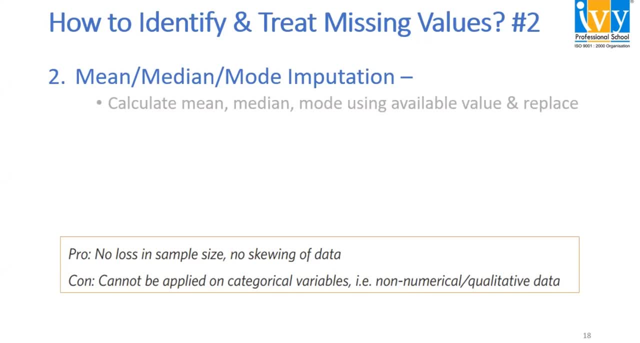 calculate mean, median mode using available value and replace mean, commonly known as the average function that we use. median is the middle value in the range of the value, and mode is the value which occurs most often in the range. Now let's see how to apply this in our data set. 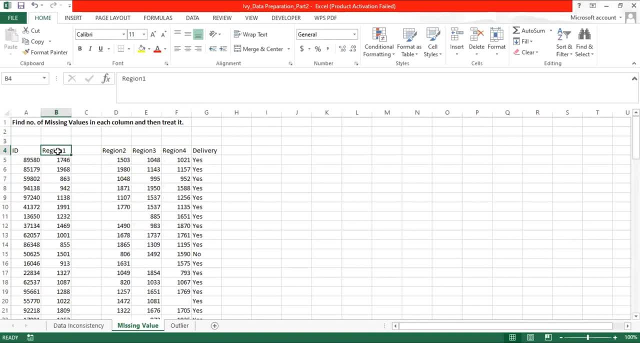 So let's insert a new column Over here and see, I want to Apply me on this data. So what I'll do is I'll convenience and just copy This column To this area and show you So when I select this. 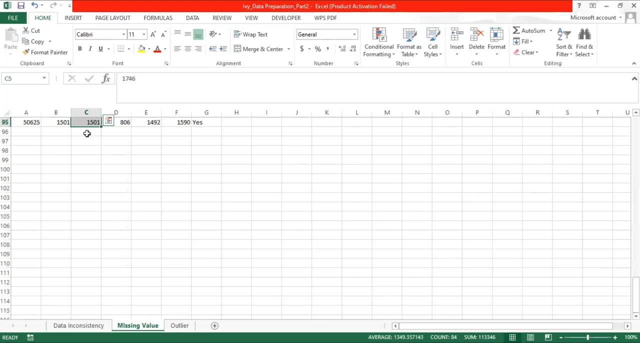 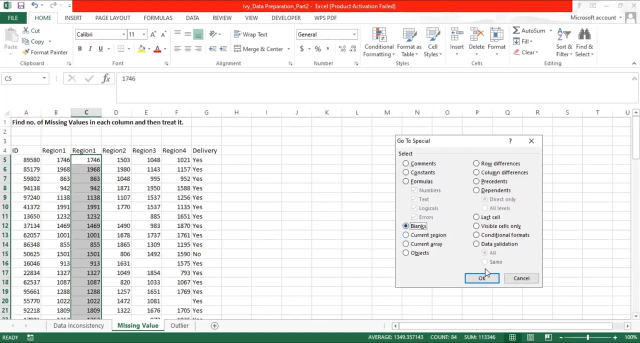 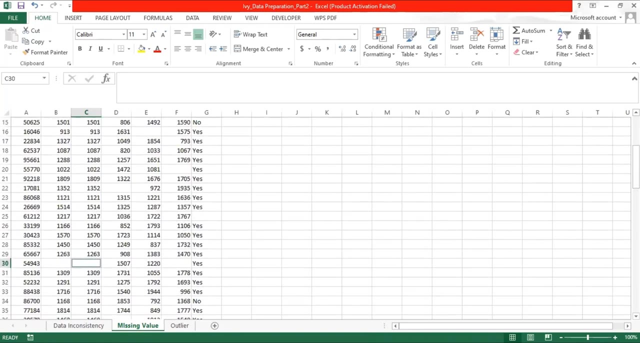 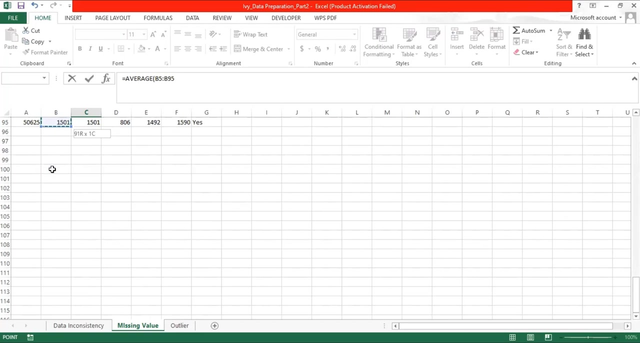 I'll fill The mean over here. I'll use control G, Go to special, Go for blanks, And the blanks will appear. Now I'll use equal to Average And select the range from your, for just convenience And fix it. 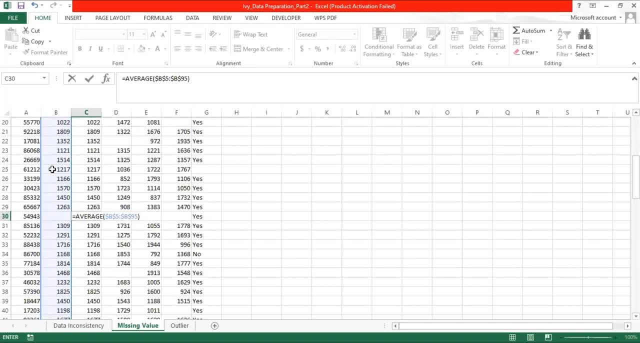 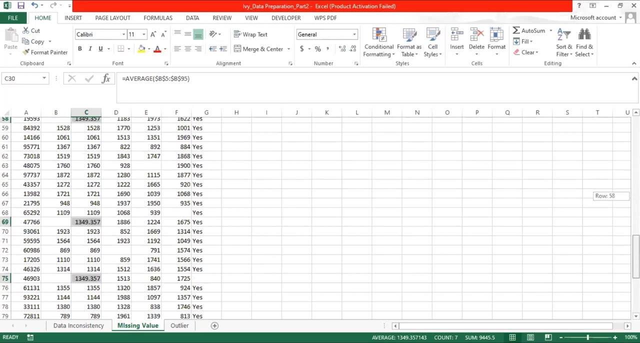 Once I do that, I'll press control enter and after pressing control enter, it will automatically Fill all the blank sets, As we can see, All these blank cells Having built with the mean. So this was the way how we can use the mean. 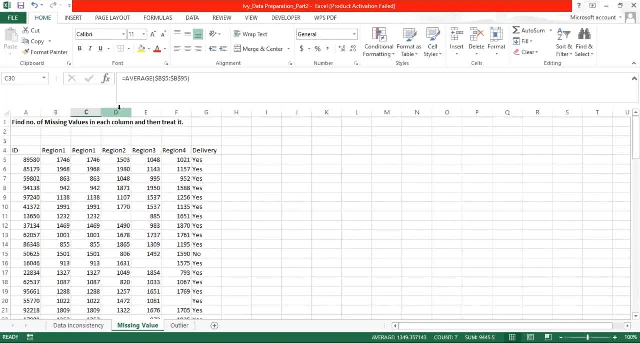 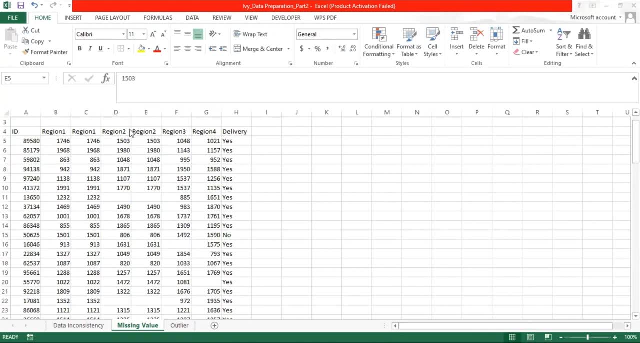 To fill up and replace the missing data. Now let's take another example and use median. Now I had created a copy column of region two over here, just for seconds it. what I'll do is similarly, in a very similar way as I did, in mean, I'll select the whole column.